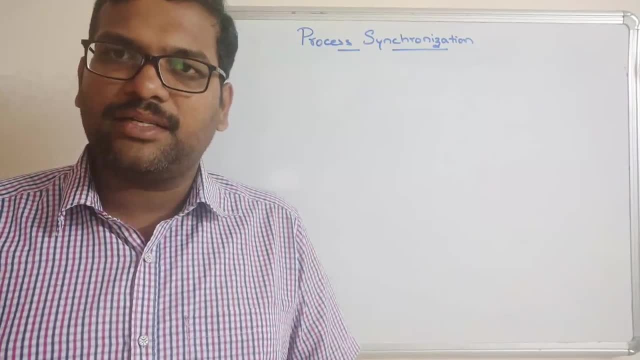 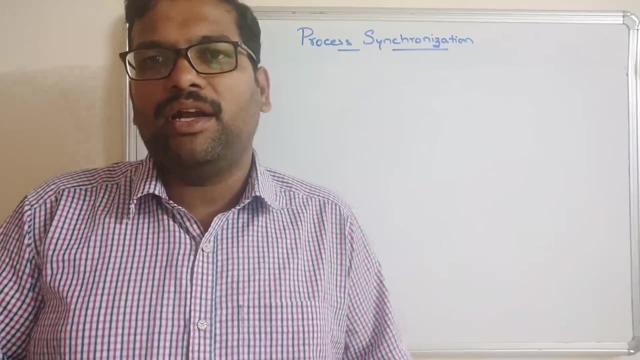 can have multiple threads and there are different types of threads: kernel threads, kernel threads and user threads. So at a time multiple threads can be implemented concurrently that we call it as a multi-threading right. So here, if two process- I mean here there are- 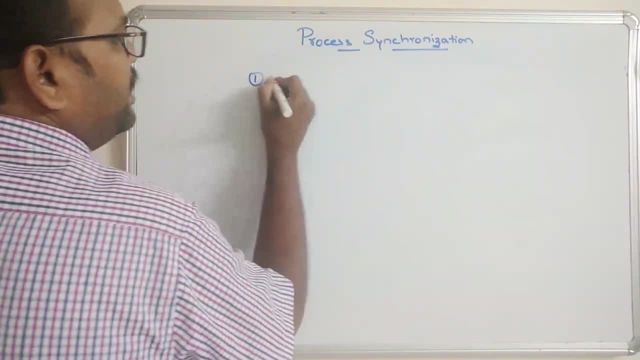 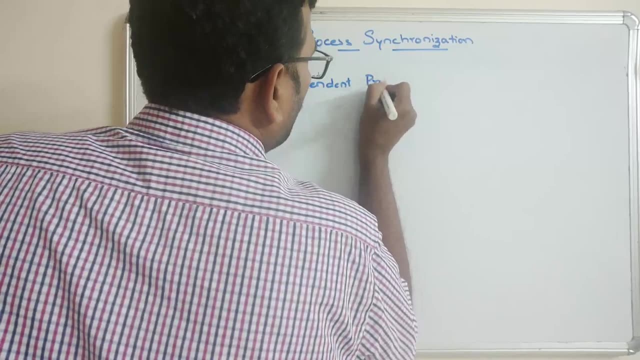 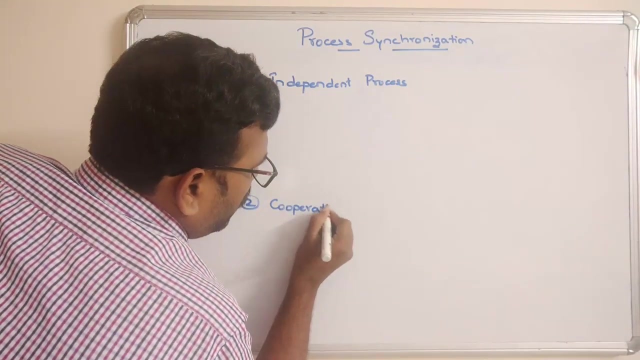 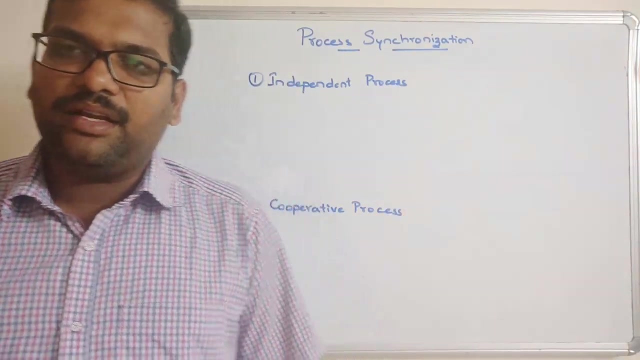 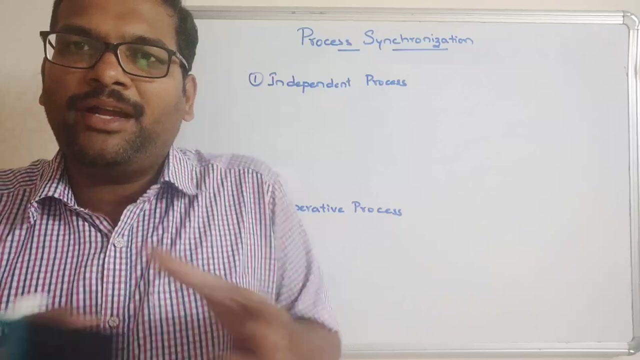 two types of process, mainly So. one is independent process, independent process, and the second one is cooperative process. cooperative. So, coming to the independent process, the name itself indicates So if one process is being executed, so that all the resources required by that process will be bind towards that process. 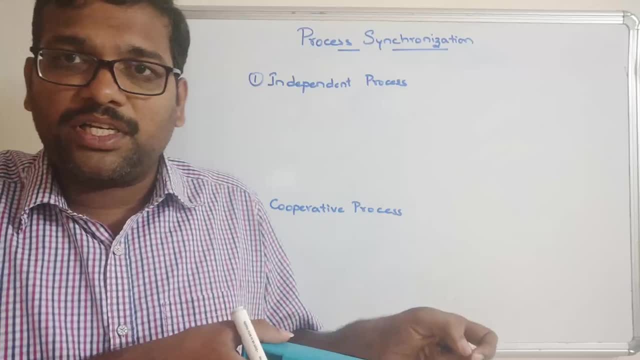 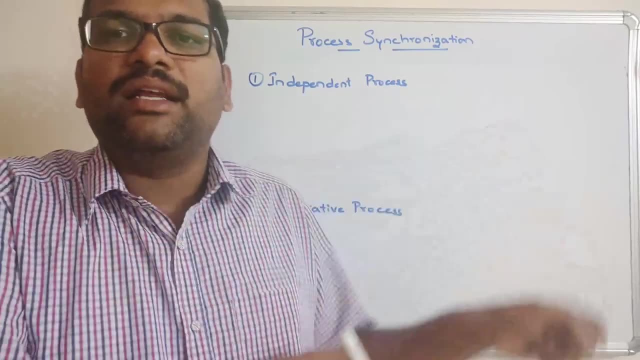 only So. that means the execution of one process does not affect the execution of another process. So once the process completes its execution, then only the resources will be released and those resources will be associated with the other process. So if one process is being executed, 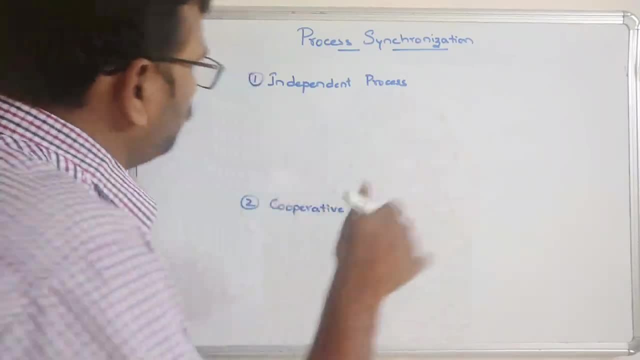 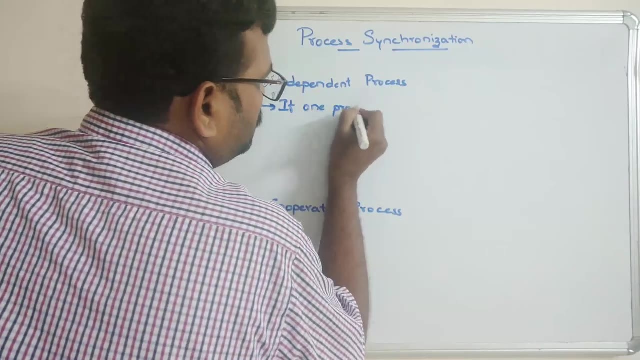 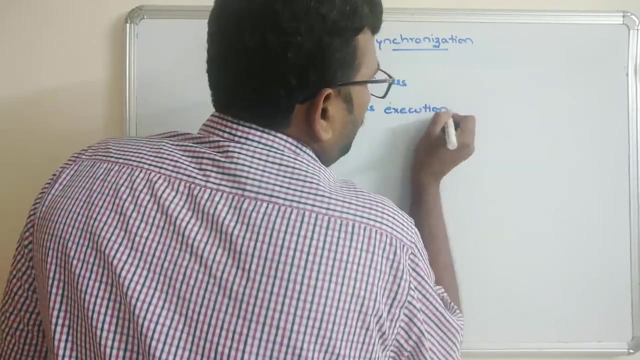 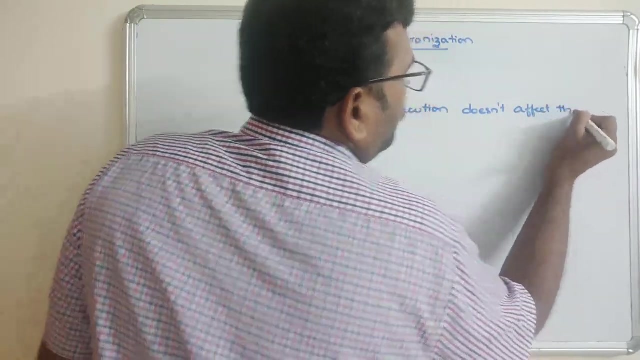 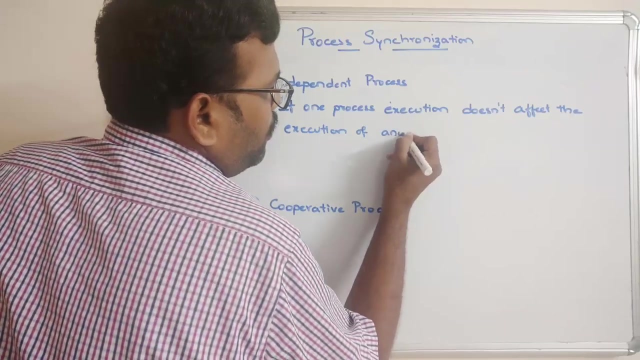 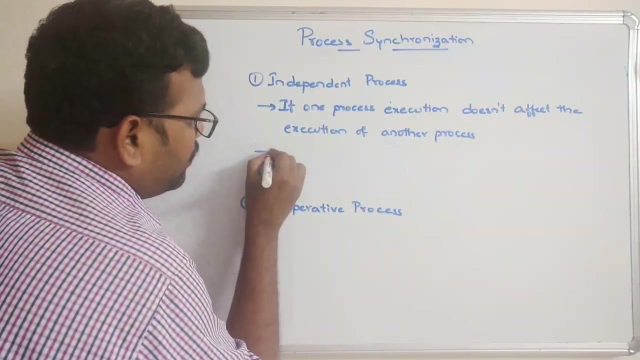 the other process. So that is why we call it as an independent process. So if one process, one process execution does not affect the execution of another process, another process, then we call it as an independent process. And here no shared memory, no shared. 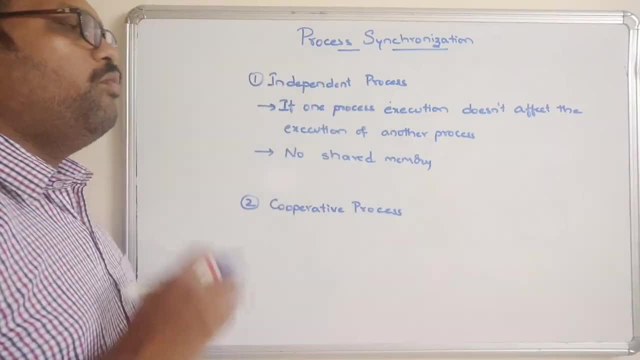 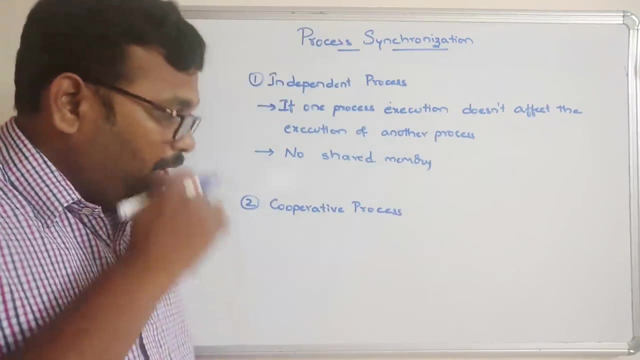 memory right. So once it was executed, then only it will move on to the next process. The execution of next process will be started. But that does not happen in the cooperative process. So in this cooperative process we call it as an independent process. So 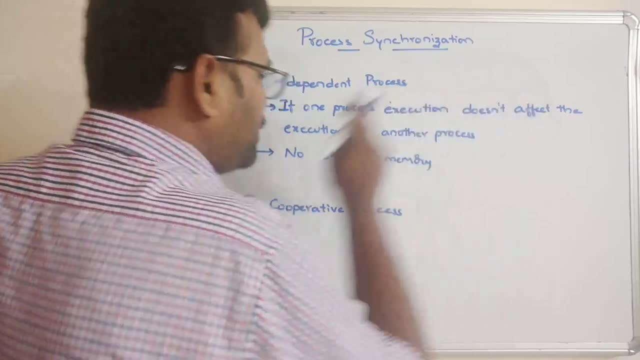 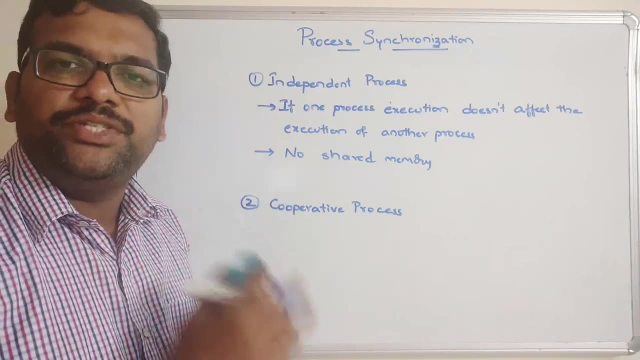 once it is executed, then only it will move on to the next process, The execution of next process. one process execution affects the execution of another process, because here, in this cooperative process, the memory will be shared memory, So one memory will be shared. 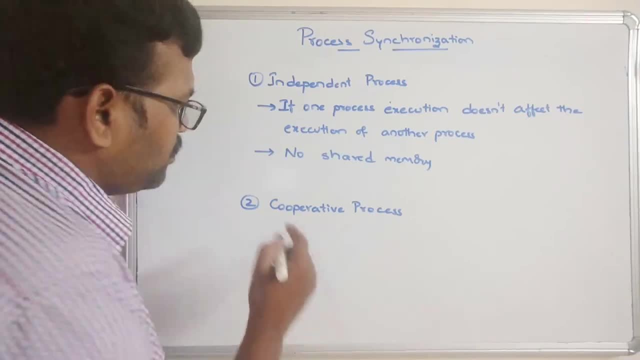 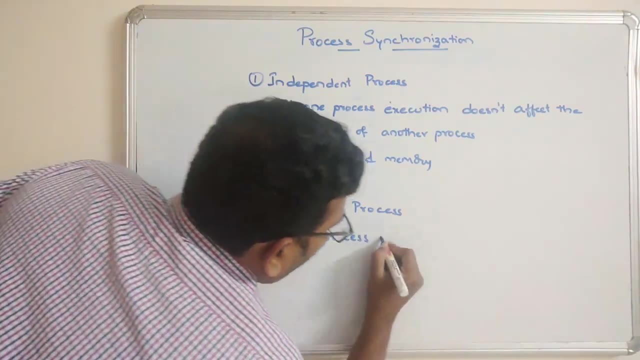 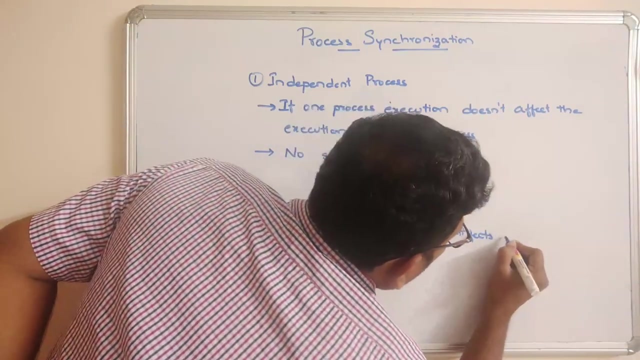 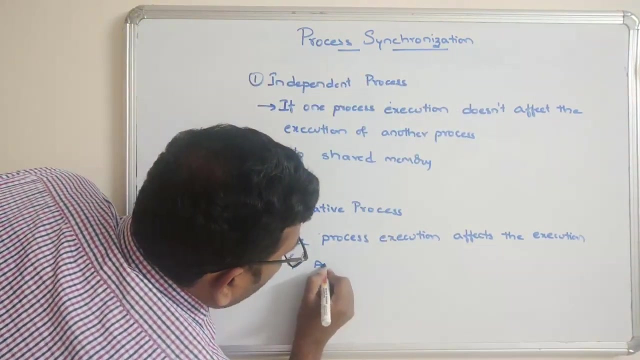 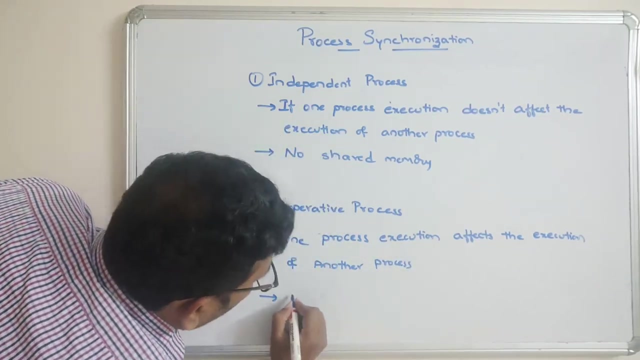 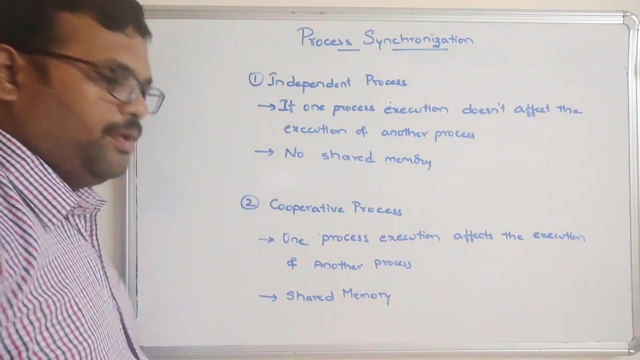 among different processes, right? So the first point: one process execution. one process execution affects the execution of another process, another process, And here there will be a shared memory, shared memory. okay, The memory will be shared memory. So here, in this particular, 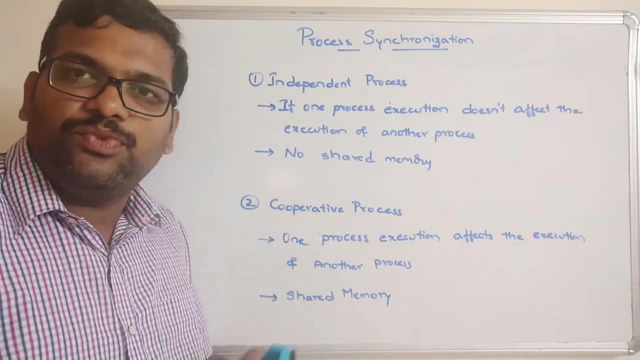 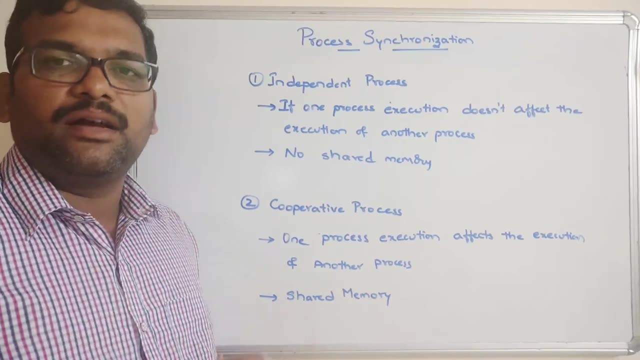 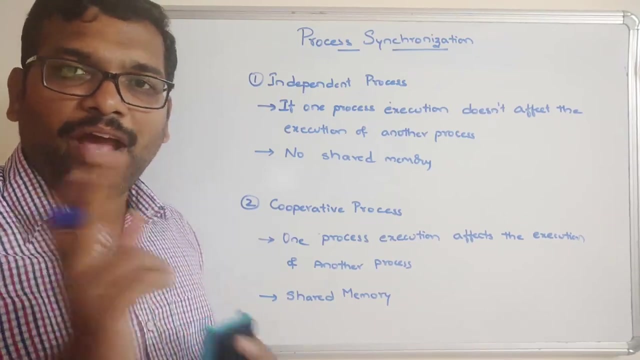 cooperative process, so multiple processes will be executed. So one process execution affects the execution of another process and multiple processes will share the common memory. So if multiple process shares the common memory, then the problem occurs with the data. So there might be a chance of getting inconsistent data. So in order to avoid that, 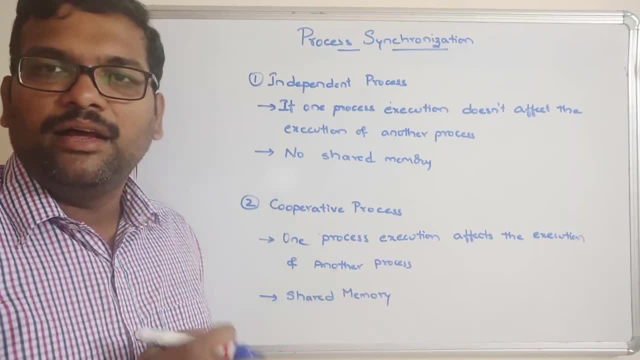 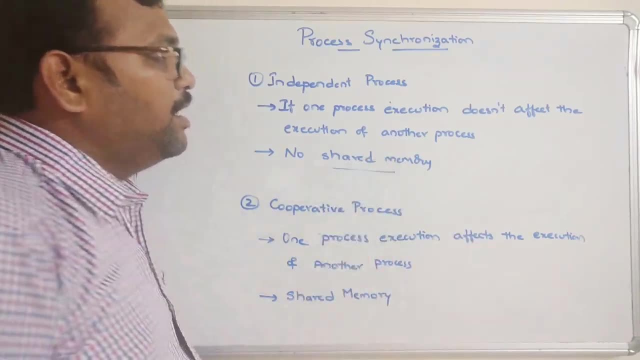 inconsistent data and to maintain the data consistent we have to follow this process: synchronization. And here we are not using initial memory. So here the process. synchronization is does not require, So here we are not using initial memory. So here the process. 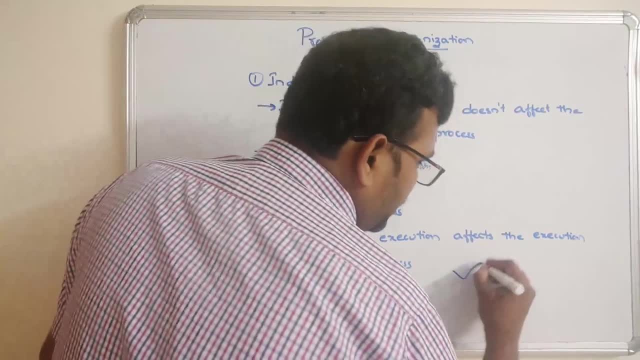 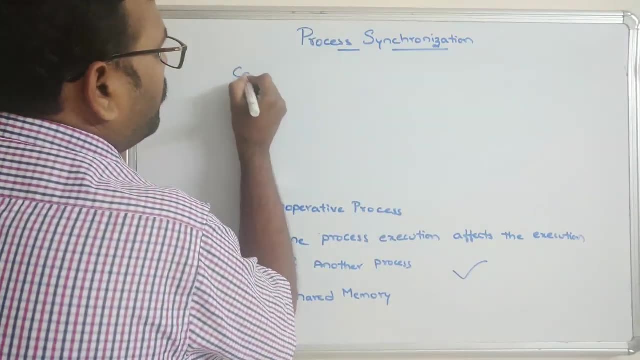 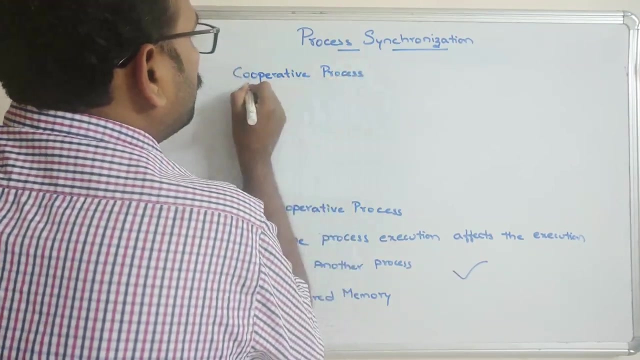 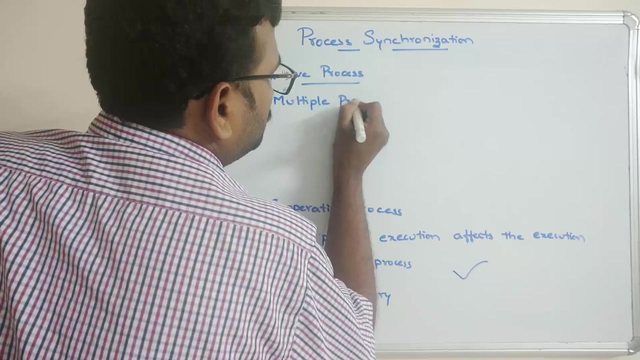 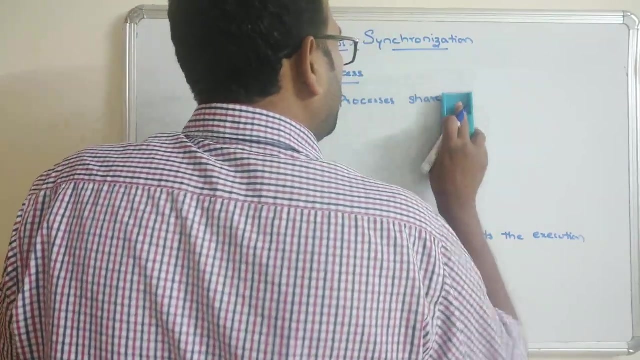 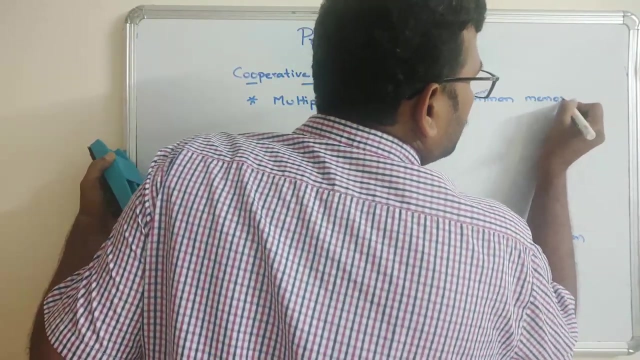 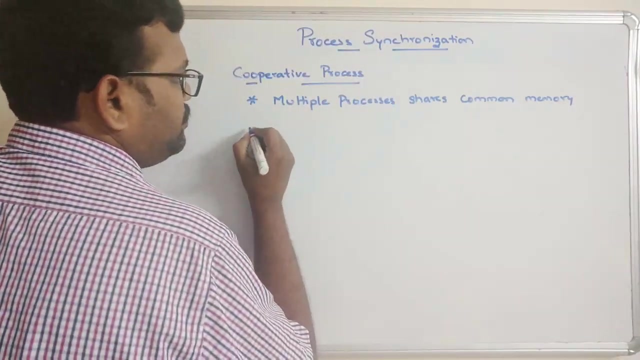 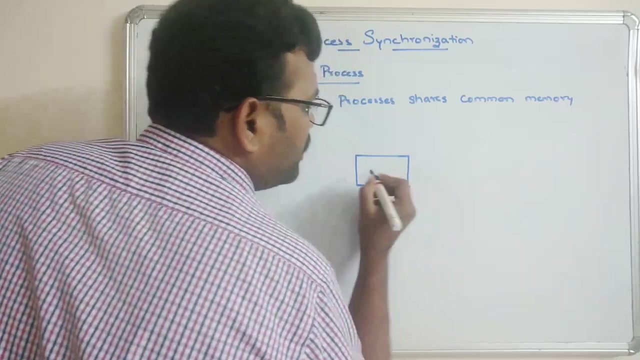 right. but in the cooperative process, the process synchronization must be there, right so our problem with cooperative processes, our problem with cooperative processes, right so here, multiple processes shares a common memory shares common memory. so let me tell you one simple example. common memory, so let it be. this is a memory, so, which is having some value. 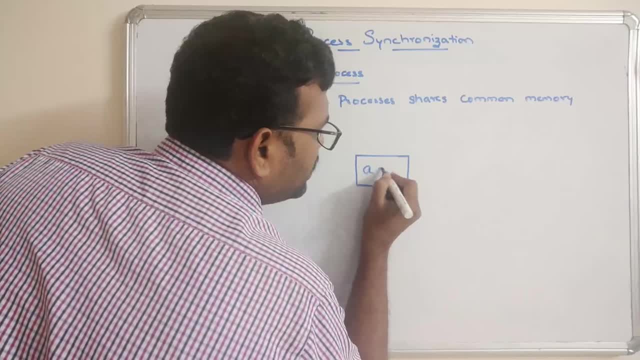 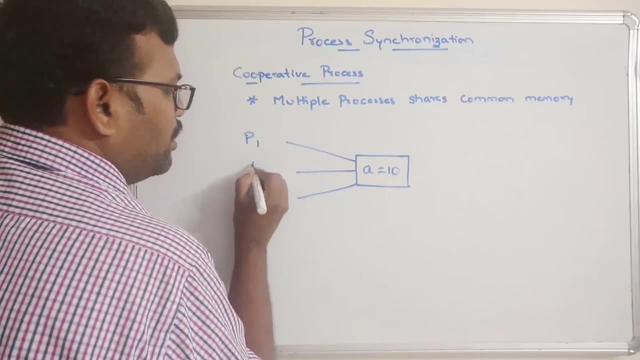 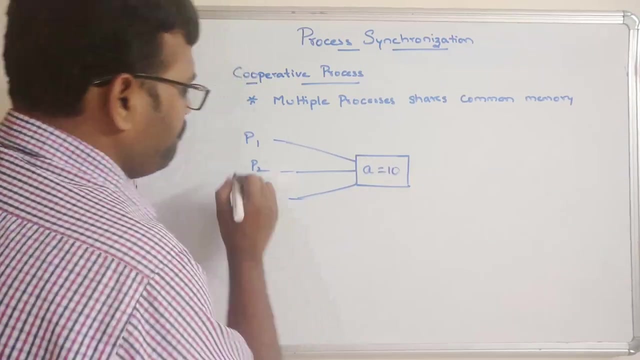 some variable, a common variable. some a is equal to some ten, so it is associated with the different processes. so let it be p1, p2, p3, so all the three process want to share the same memory. common memory and p1 will be as follows: 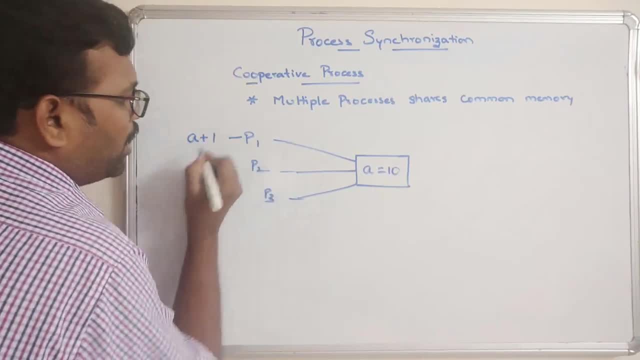 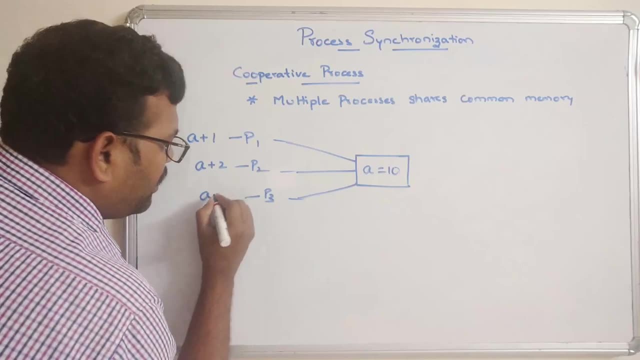 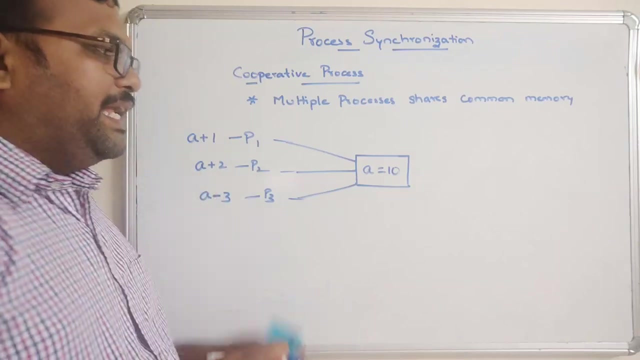 wants to update A with 1, P2 wants to update A with 2, P3 wants to, I mean, update A with negative 3, okay, so A plus 1, A plus 2, A minus 3, if all the three processes shares. 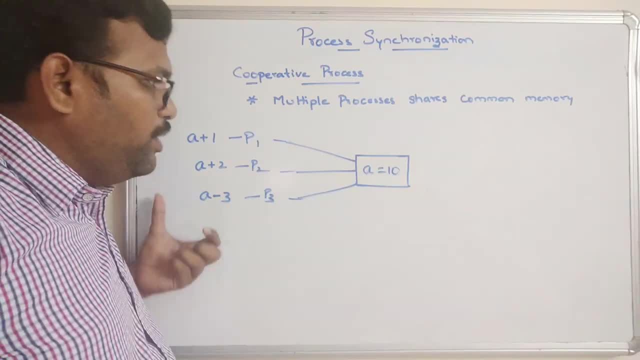 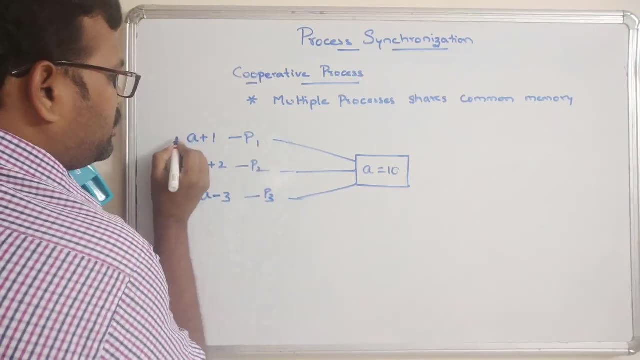 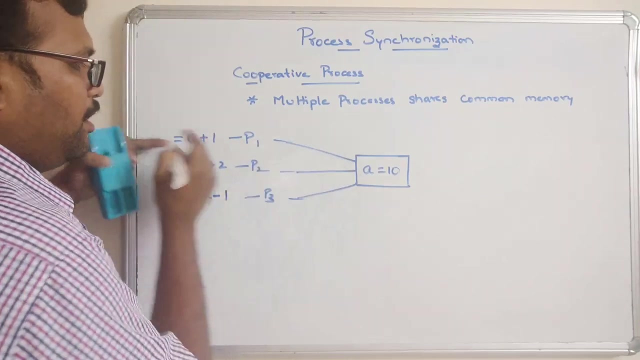 the same memory. if all the three want are doing the same operation at a time. what happens here? so if P1 is started, the executing P1 will be having, for example, here I will go with the 1, so P1 will be having. what is the value of this one after executing? 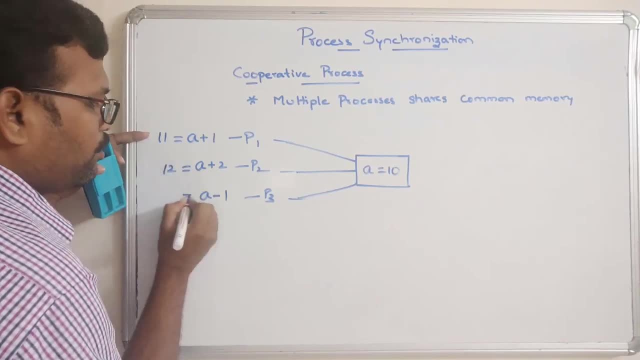 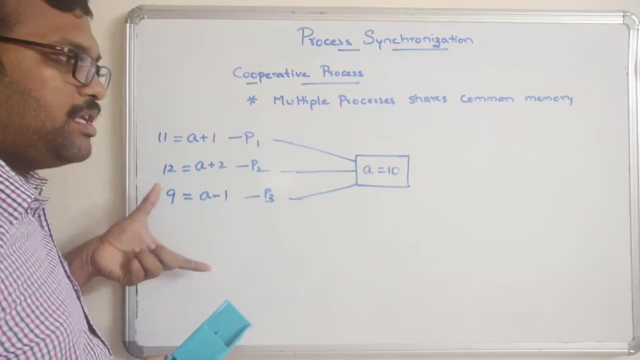 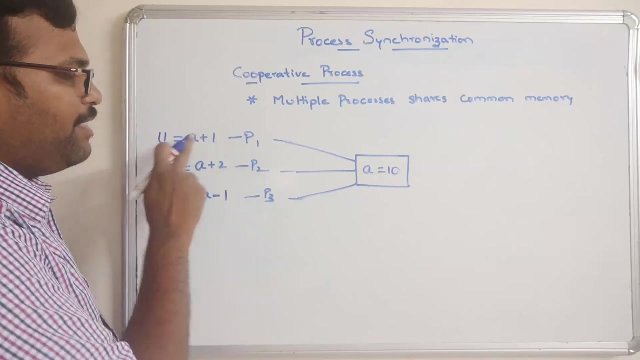 P1,, 11,, 12,, 9,. right, so all the three processes are sharing the common memory and all the three processes are doing the same job at a time at once, right? so, according to the process, for P1, A value is 11,. according to P2,, A value is 12,. according to P3, A value 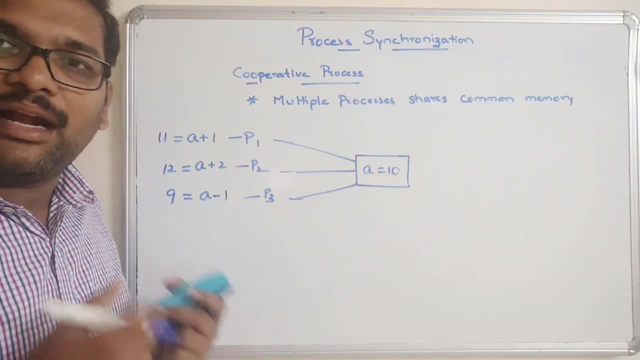 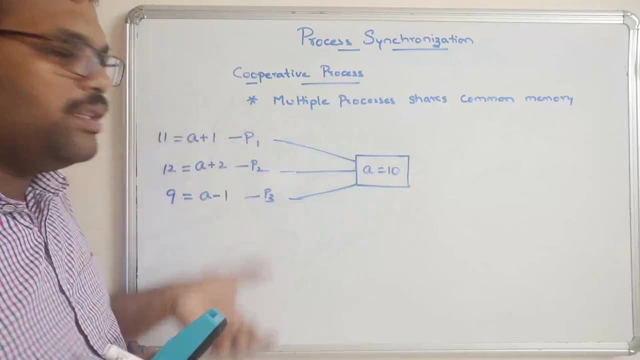 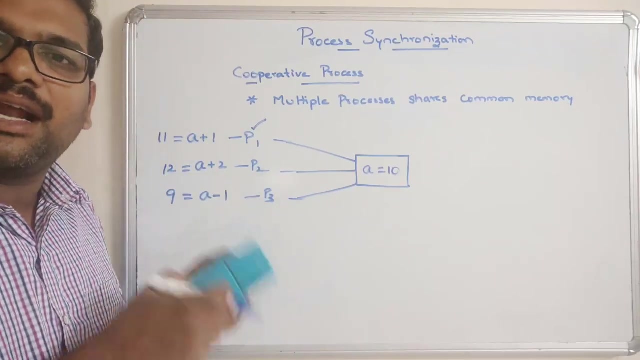 is 9, right. so which one is the correct result? which one will be the correct result? because A is the common variable which is being shared among all the different processes. so here, P1 tells that. so P1 itself is the correct value. P2 says that P2 itself is the correct. 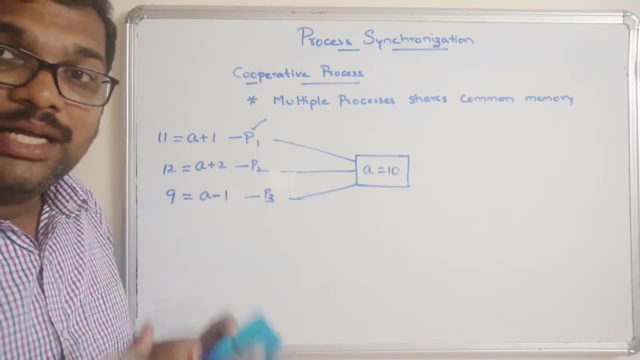 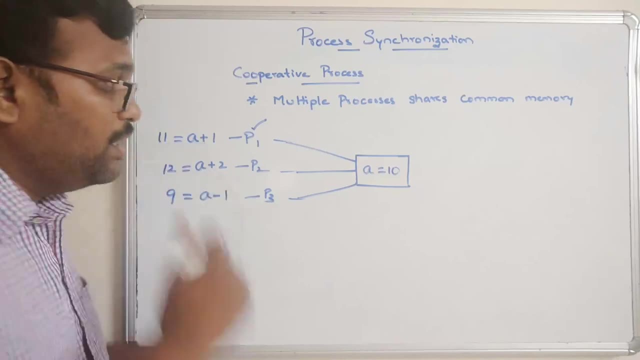 value. P3 says that P4 is the correct value, P5 is the correct value, P6 is the correct value, so P3 itself is the correct value. so some sort of race is going on telling that the process is having the correct result. so such a situation, such a situation is called. 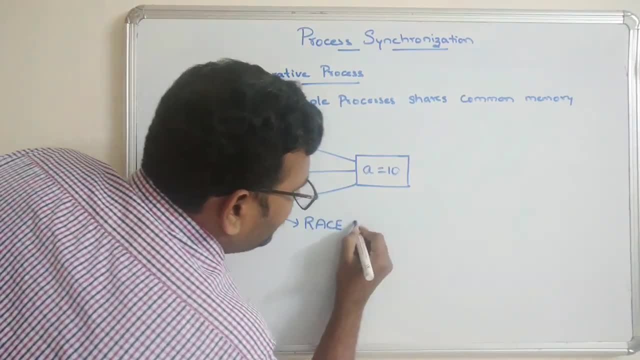 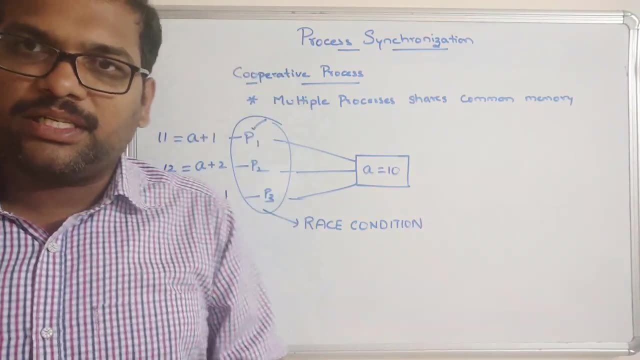 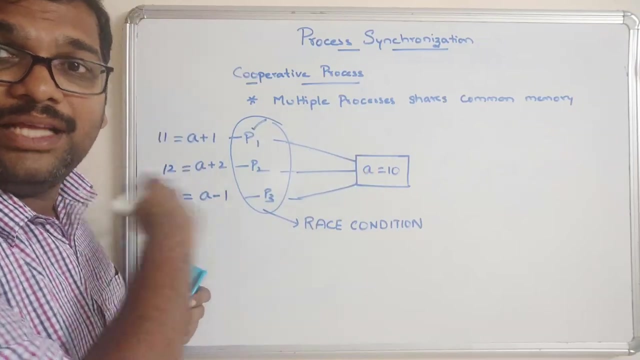 as race condition, race condition. so if there is a in particular, this cooperative process, so there is an inconsistency of data. so, according to one process, there is an inconsistency of data. so according to one process, the value of A is changed. right, so this, this, 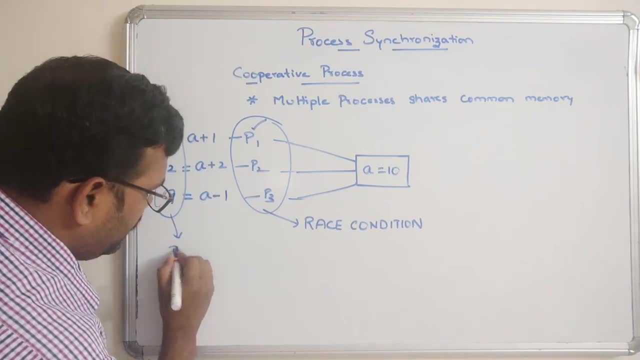 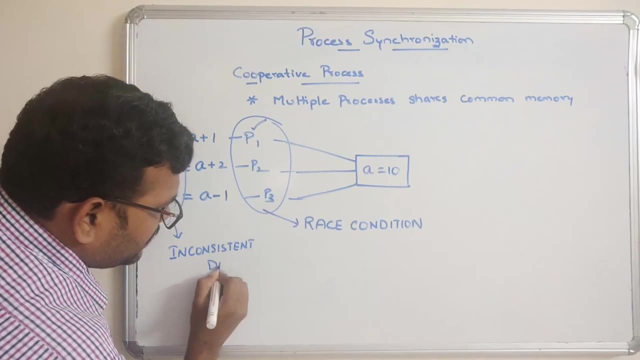 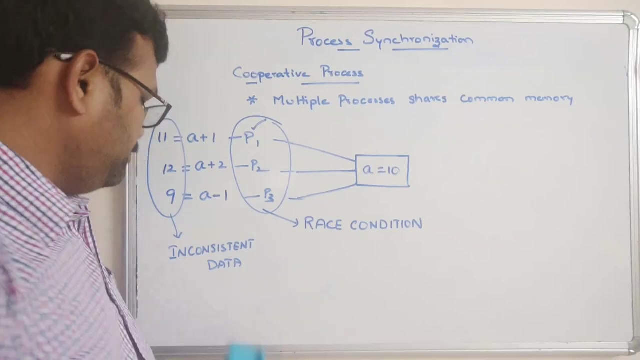 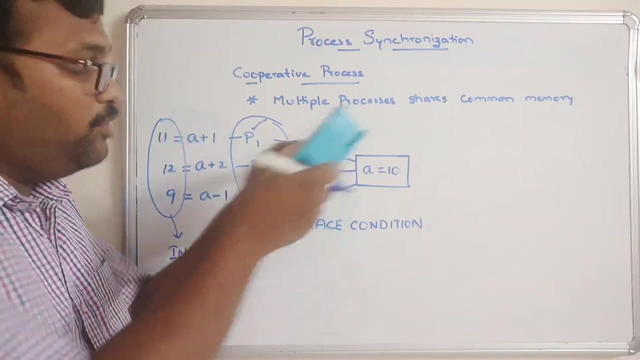 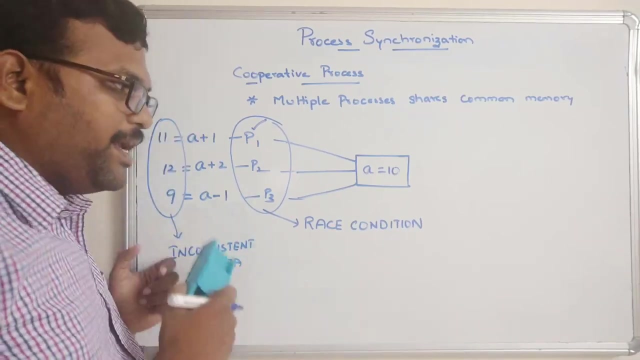 is called. this is called inconsistent data. inconsistent data, so that should not happen. right, that should not happen. so we have to make this one as a consistent data. so same value should be Available for all the three processes so that for that consistent data making of 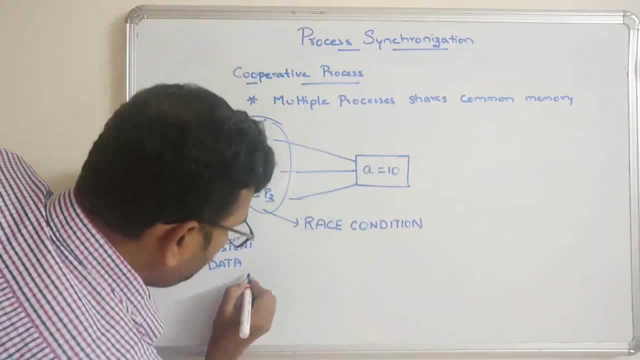 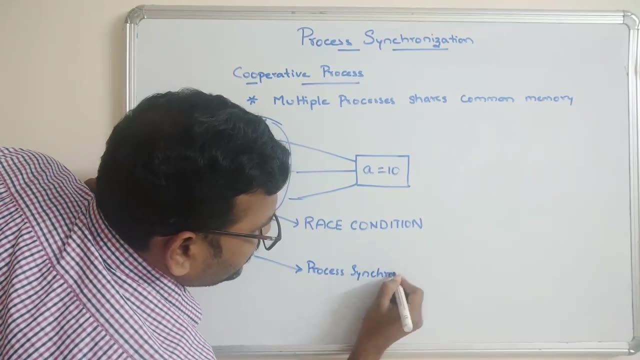 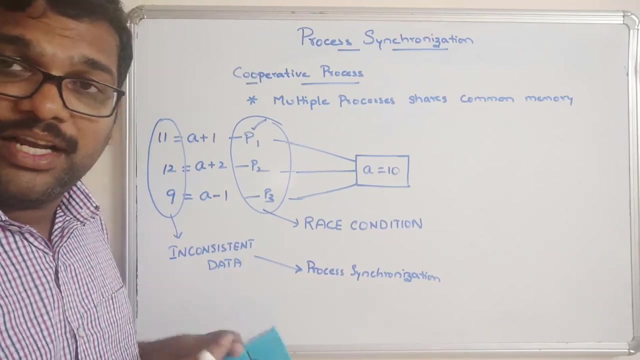 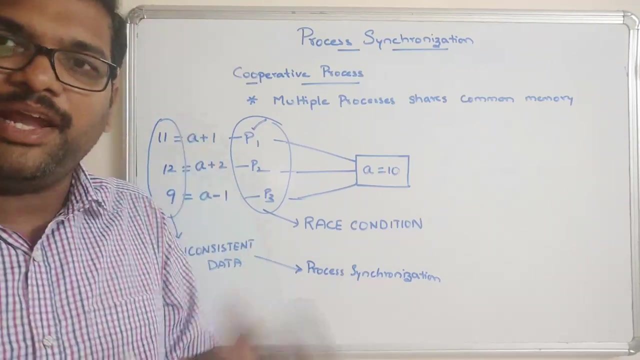 this one to consistent. we are moving with process synchronization, process synchronization, so where some locking system will be there. if one process is executing the shared memory right, so automatically the remaining Process have to wait until the process completes its execution. so then the common variable. 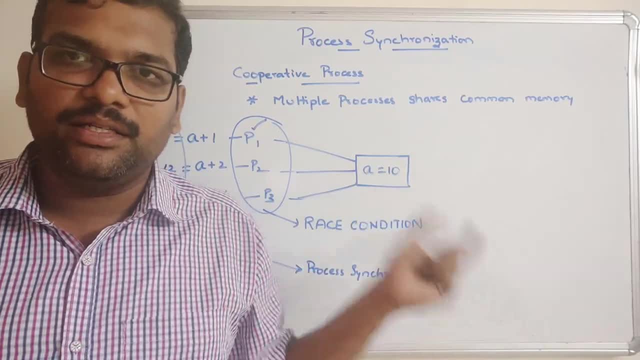 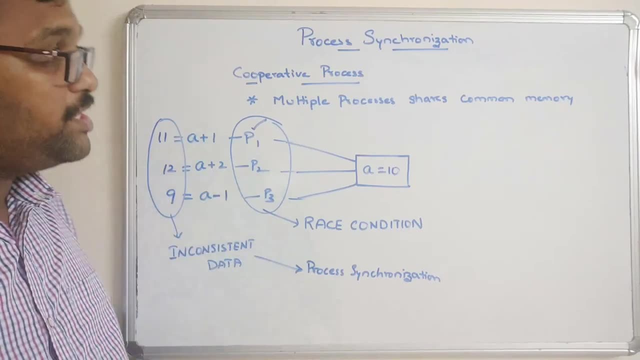 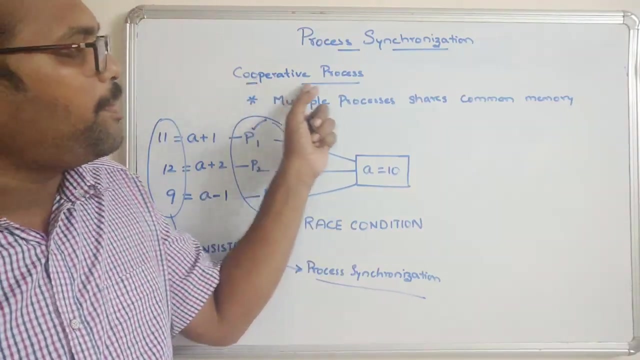 will be having the consistent data. the shared memory is. I mean the memory is shared among different process, so with a consistent data right. so in such a situations we are moving with this process synchronization. so the main problem is this type of process cooperative. 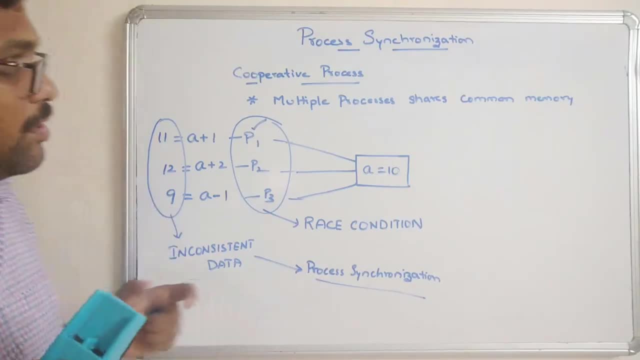 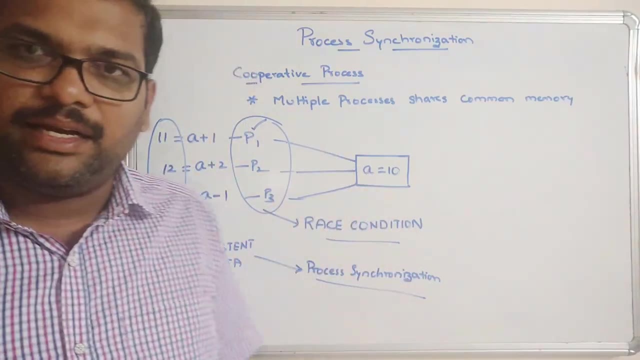 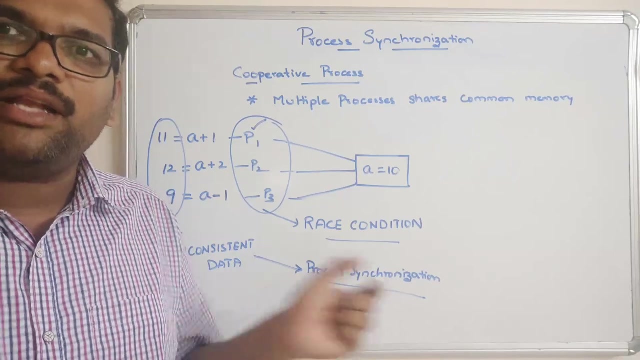 process. okay, so let us stop here. Hope you understood this race and decision. because of inconsistent data and in our next session we will see about the few problems so that may require this process synchronization, If you are having any doubts regarding this one, feel free to post your doubts in the 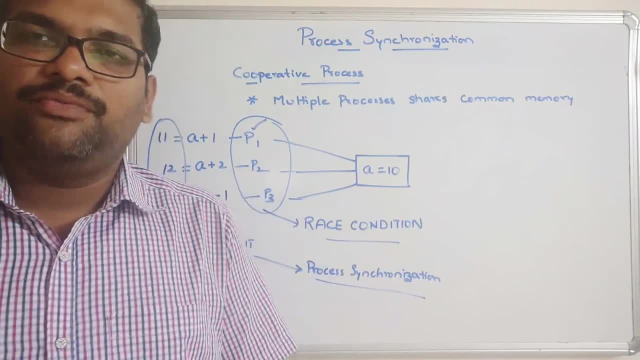 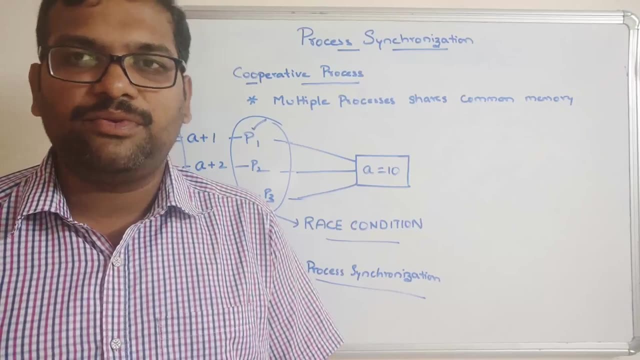 comment section. definitely, I will try to clarify all your doubts. If you have really enjoyed my session, like my session, share my session with your friends and do not forget to subscribe to our channel. thanks for watching. thank you very much. Bye, bye.